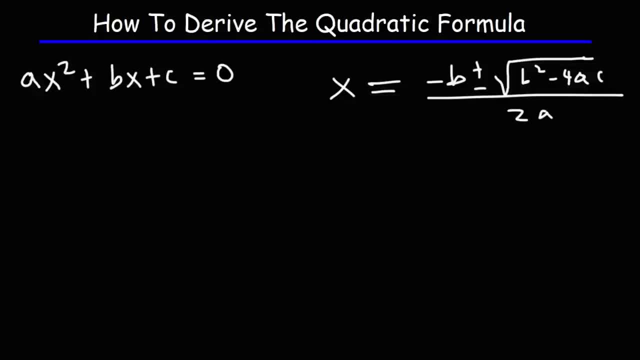 In order to derive that formula, what we need to do is we need to solve for x, And we have to complete the square in order to do so. So let's get rid of this to make more space. The first thing I'm going to do is I'm going to take the constant term c and move it to the other side of the equation. 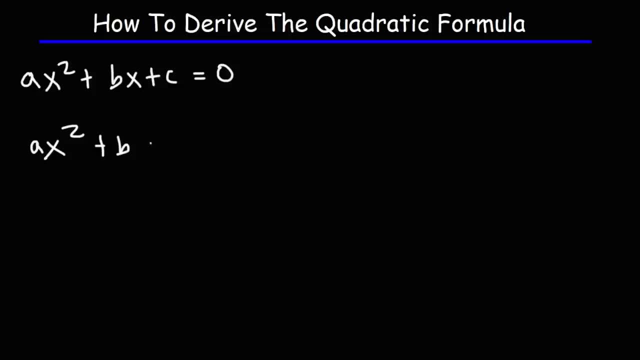 So we're going to have ax squared plus bx. Leave a square root of bx. Leave a square root of bx. Leave a space equals negative c. Now the next thing that we need to do is divide everything by a, So a will cancel here. 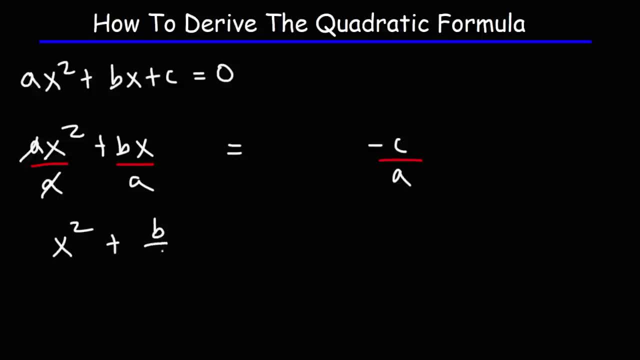 We're going to have x squared plus b over a times x is equal to negative c over a. So now, at this point, we need to complete the square. In order to do that, we need to take half of that coefficient, b over a. 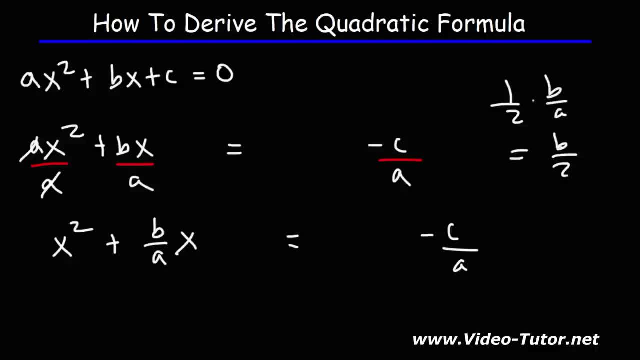 One half times b over a is b over 2a, So we're going to add that to both sides of the equation. But we need to square this result. So we're going to add plus b over 2a, squared. Whatever you do to the left side, you must also do to the right side. 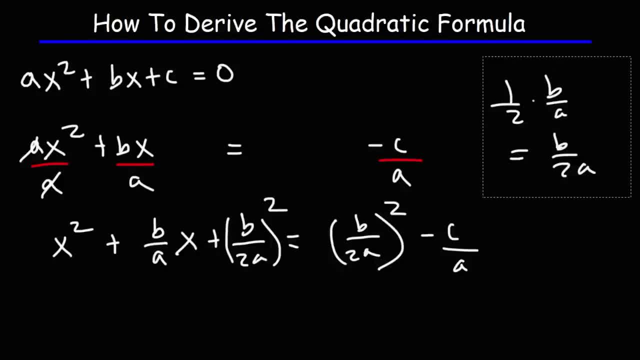 So that the value of the equation is going to be b over 2a squared, So that the value of the equation on both sides of the equation remain the same. So now, at this point, we need to factor the perfect square trinomial that we have on the left side. 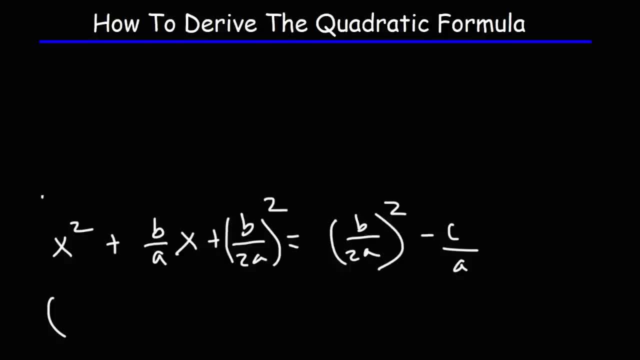 A quick and simple way to factor a perfect square trinomial is to follow these steps. It's going to be x, whatever variable you see there, and then whatever sign you see here, plus Whatever is here before it's squared. So x plus b over 2a squared. 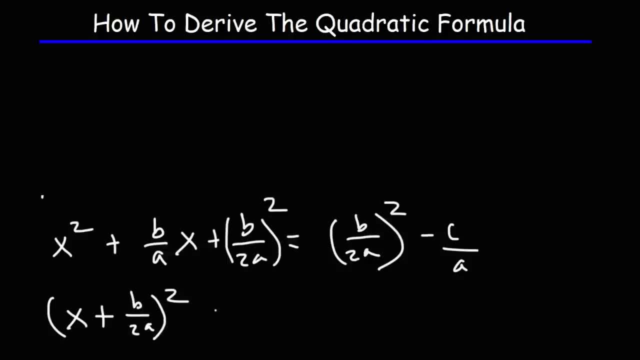 That's a very quick and simple way to factor a perfect square trinomial On the right side. we can go ahead and square that term. So it's going to be b squared over 2a squared is going to be 4a squared. 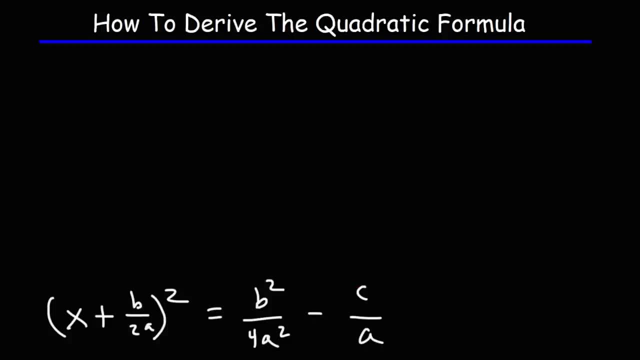 Now the next thing that we want to do is we want to convert This expression from two fractions into one fraction, And so to combine two fractions into one, you need to get common denominators. Therefore, we're going to multiply the top and bottom of c over a by 4a. 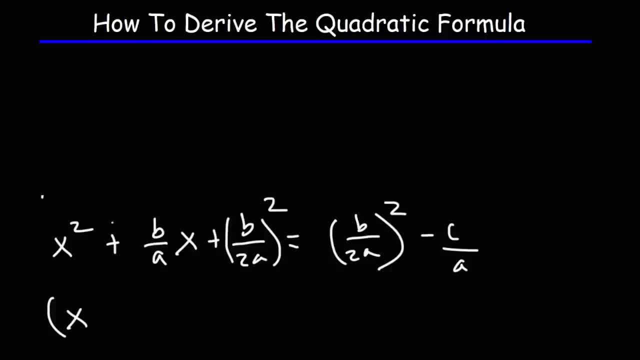 It's going to be x, whatever variable you see there, and then whatever sign you see here, plus Whatever is here before. it's squared. So x plus b over 2a squared. That's a very quick and simple way to factor a perfect square trinomial. 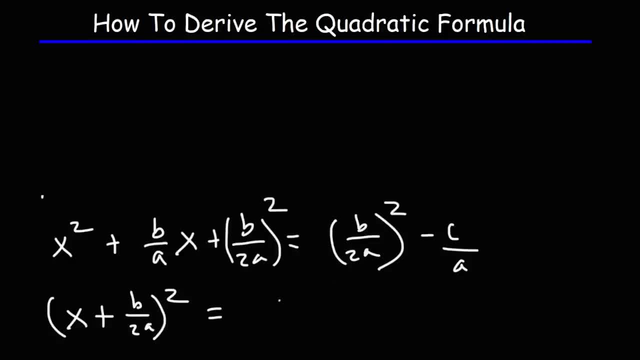 On the right side. we can go ahead and square that term. So it's going to be b squared over 2a squared is going to be 4a squared. Now the next thing that we want to do is we want to convert. 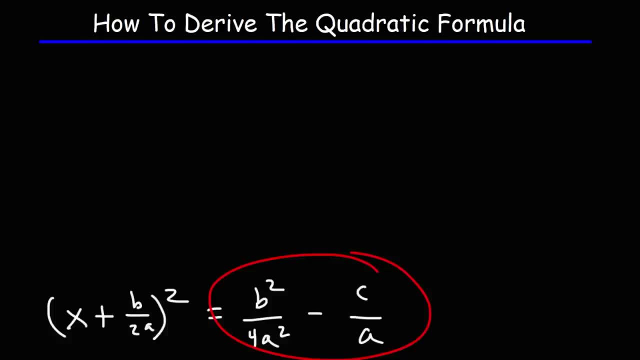 This expression from two fractions into one fraction, And so to combine two fractions into one, you need to get common denominators. Therefore, we're going to multiply the top and bottom of c over a by 4a, So we're going to have x plus b over a. I mean b over 2a. 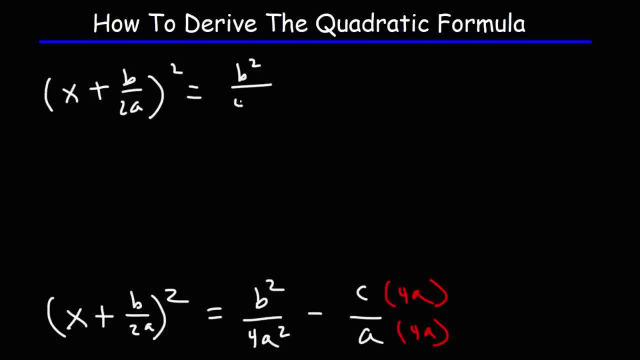 squared and that's going to be equal to over 4a squared minus. so we have 4ac over 4a squared. So now that we have common denominators, we can combine it into a single fraction. So this is going to be b squared minus 4ac, all over 4a squared. 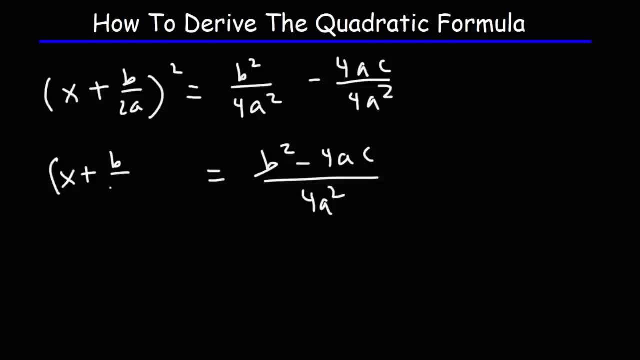 Now, what do you think is the next thing that we need to do at this point? Remember, our goal is to isolate x. We need to solve for x, So what we need to do is take the square root of both sides. The square root and the square will cancel, and so we no longer need to write the parentheses, So it's simply going to be x. 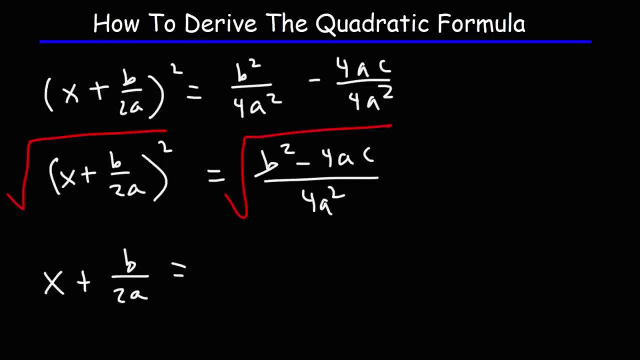 plus b over 2a, And then that's going to be the square root of b squared minus 4ac, Now the square root of 4a squared. we could simplify that The square root of 4 is 2.. The square root of a squared is 8.. 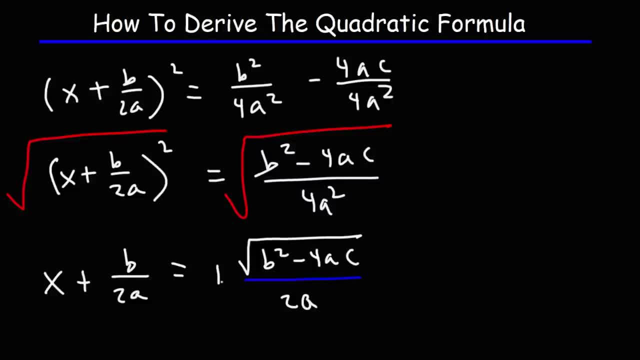 Now, because we took the square root of the right side, we can add plus or minus. The next thing we need to do is subtract both sides by this term, or simply move it from the left side to the right side. It's positive on the left side, but it's going to be negative on the right side. 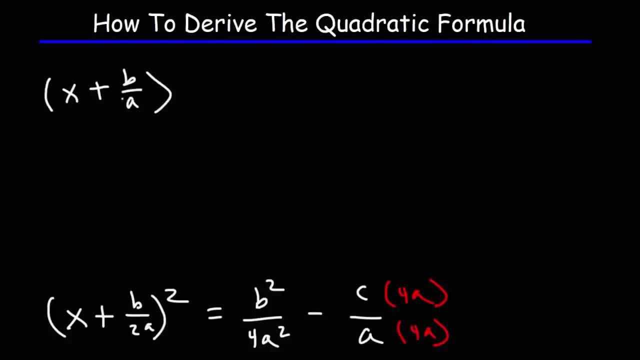 So we're Gonna have x plus b over 2a squared And that's going to be equal to b squared over 2a squared over 4a squared minus. so we have 4ac over 4a squared. So now that we have common denominators, 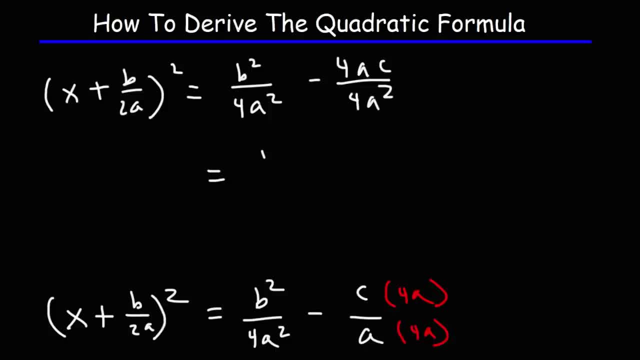 we can combine it into a single fraction. So this is going to be b squared minus 4ac, all over 4a squared. Now what do you think is the next thing that we need to do at this point? Remember, our goal is to isolate x. We need to solve for x, So what we need to do is take the 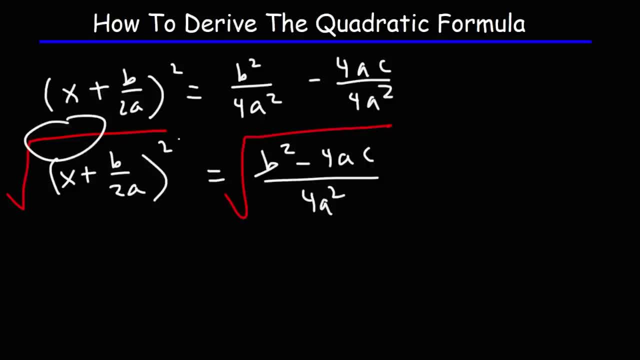 square root of both sides. The square root and the square will cancel, and so we no longer need to write the parentheses. so it's simply going to be x plus b over 2a, And then that's going to be the square root of b squared minus 4ac. Now the square root of 4a squared. 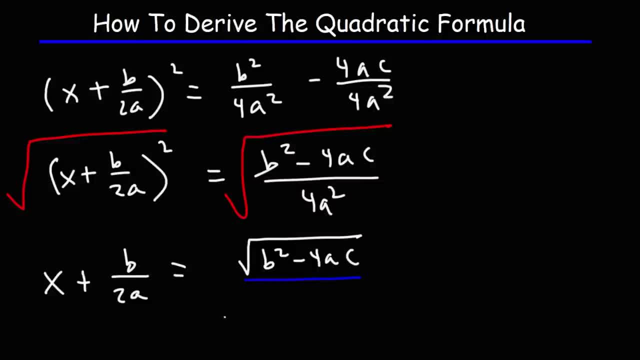 is going to be the square root of b squared minus 4ac. So that's going to be the square root of b squared. we could simplify that: The square root of 4 is 2.. The square root of a squared is 8.. 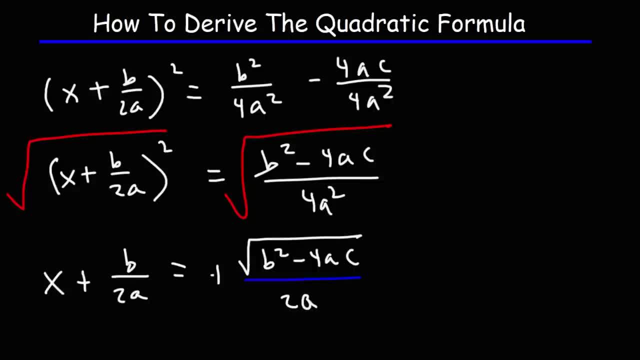 Now, because we took the square root of the right side, we can add plus or minus. The next thing we need to do is subtract both sides by this term, or simply move it from the left side to the right side. It's positive on the left side, but it's going to be negative. 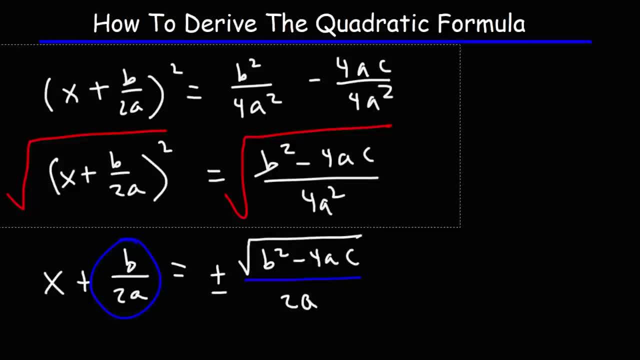 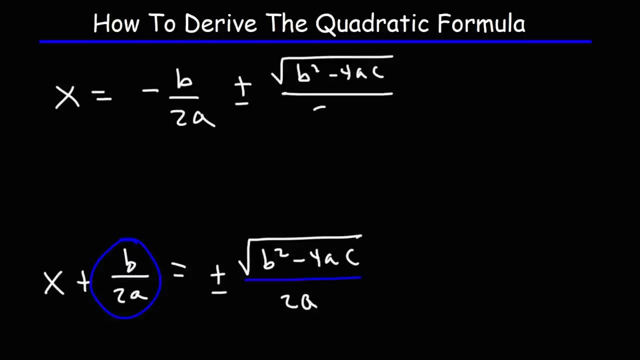 on the right side, So we're going to have to do this again. So we're going to have: x is equal to negative b over 2a, plus or minus the square root of b squared minus 4ac over 2a. Now that we have common denominators, we can combine that into a single. 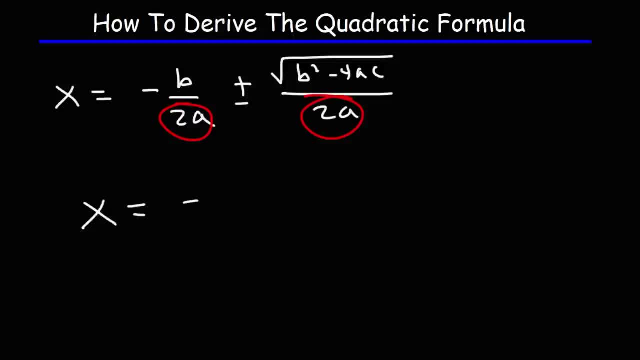 fraction. So this is going to be negative: b plus or minus the square root of b squared minus 4ac, all over 2a. And so that's how you can prove or derive the quadratic formula. starting from the quadratic equation. The key is to complete the square and then solve for x.